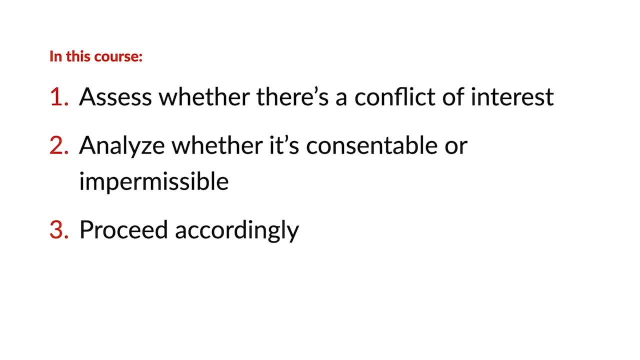 explore these steps in the context of the conflict of interest rules and their applications in the everyday practice of law. Although we've previewed the simple sounding three steps to determining whether there's a conflict, let's break it down further And I think the easiest way to understand conflicts and how they 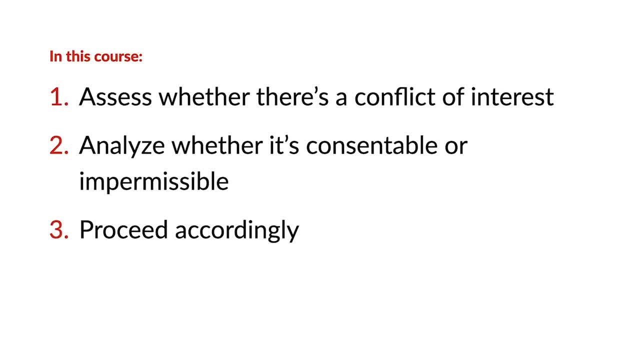 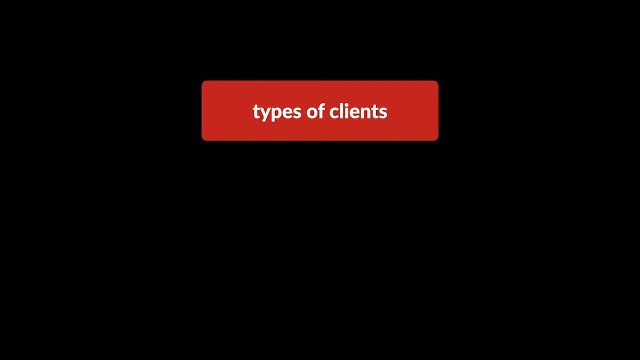 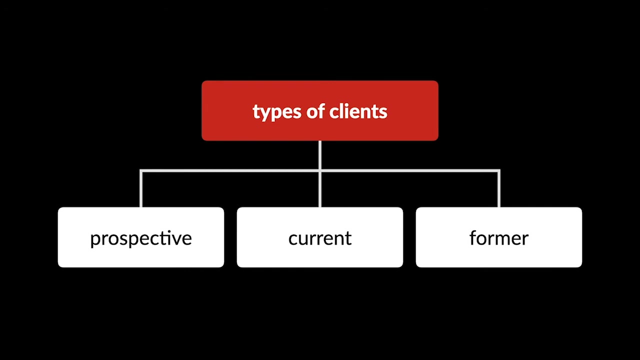 apply is to first define the type of client that you're talking about, or rather the status of the client, And what do I mean by that? We can divide clients into three main status types: the prospective client, the current client and the former client. and depending upon which type of client, 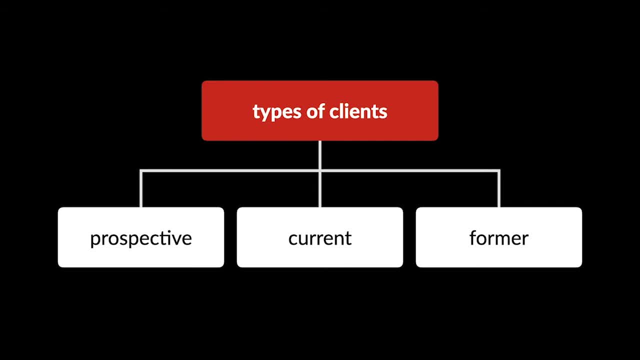 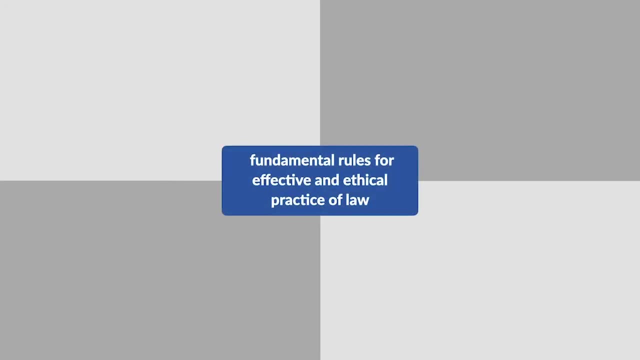 you're dealing with. the conflict rules apply somewhat differently. now we're talking about legal ethics, so before we get to the actual numbers of the conflict rules, let me just lay out to begin with, the fundamental rules for effective practice of law- effective and ethical, I usually point out- are 1.1 and 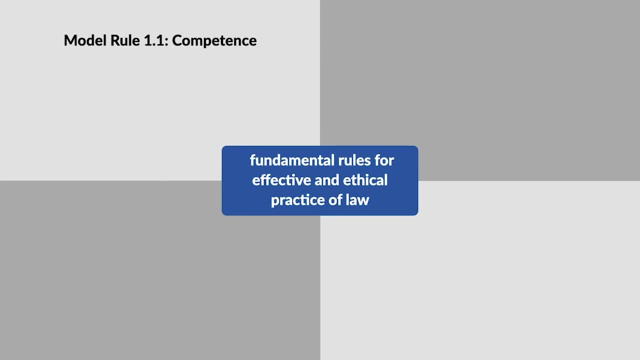 I'll be using the model rules here, which is competence, 1.3, which is diligence, and 1.4, which is communication, and 1.6, which is confidentiality. now there are many other important rules, but the bottom line is: competence tells you. you have to understand what you're doing. 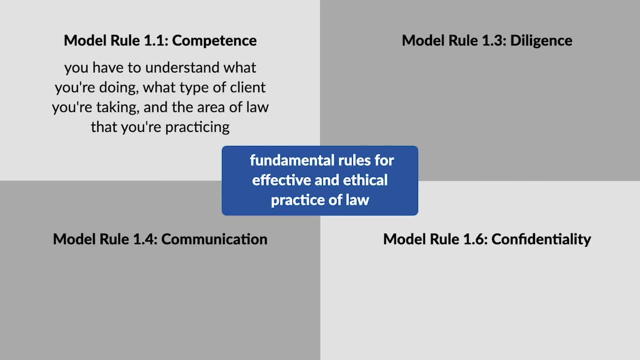 what type of client you're taking the area of law that you're practicing or be able to learn it. diligence requires you not only to remain diligence in your ongoing education in the law, but it's focused on being diligent with your clients and your clients cases, so you can see how the two kind of go hand-in-hand.